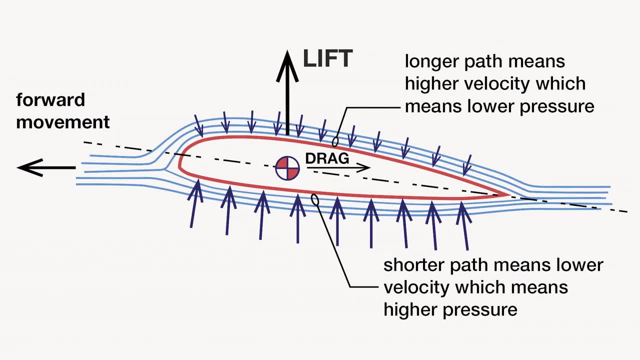 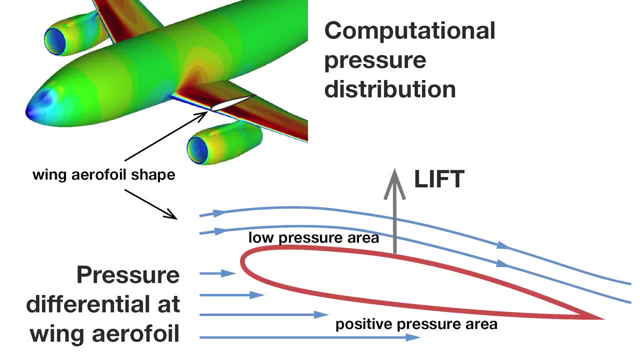 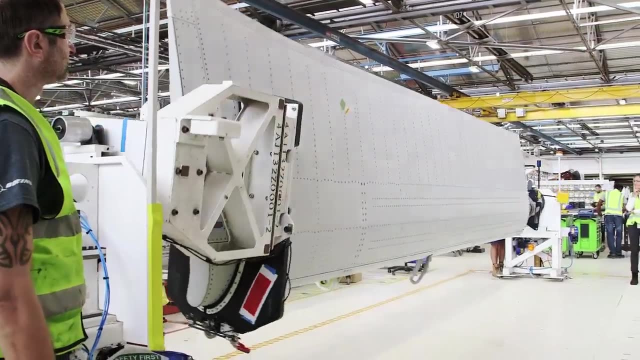 acting over the entire wing surface. It acts to deflect or bend the wing upwards. Aircraft are designed to carry a load and to resist stress. Stress is basically the amount of load that can pass through a structure per unit area. The determination of such loads. 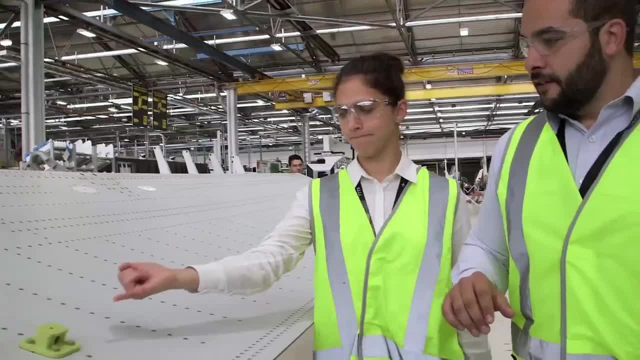 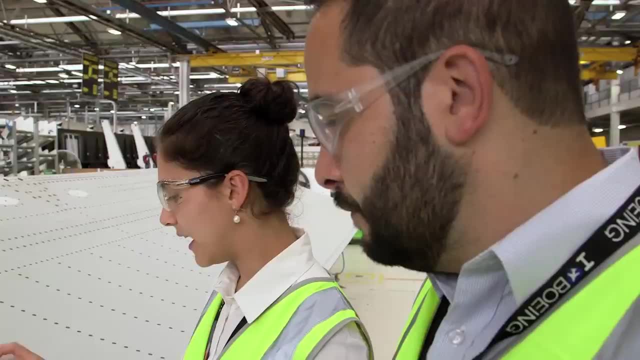 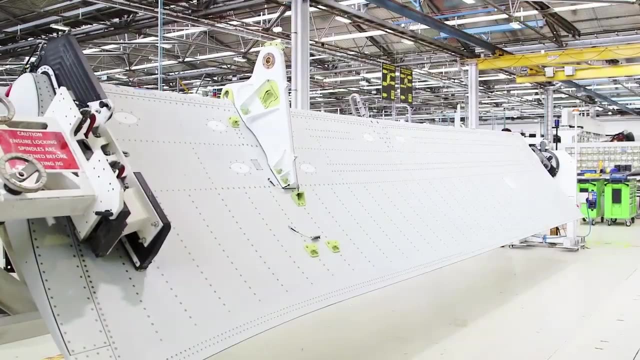 is called stress analysis. Structural engineers at Boeing Aerostructures Australia in Melbourne have to calculate the stresses involved In order to design a structure to be able to sustain a flight and to carry the loads that are expected On a day to day basis. I am looking at a part and assessing its capability for flight loads. 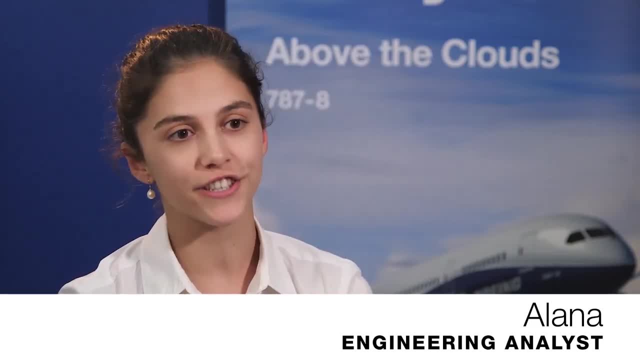 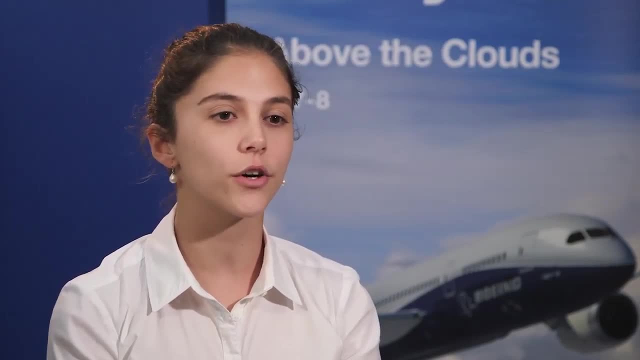 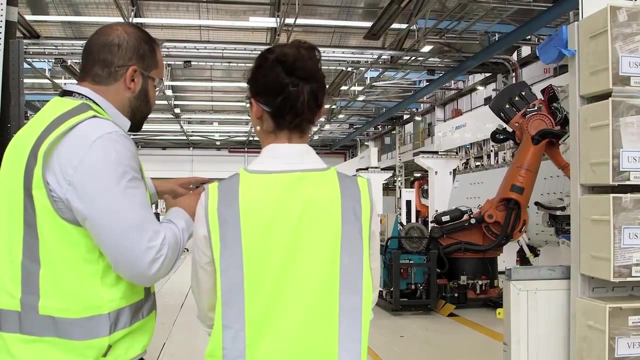 ground loads, handling loads, vibration loads, Basically, any load that the part can expect to experience in its life. on the aircraft, I am assessing it for its suitability, for One of the first things we do when we start analysing a part is we like to understand the structure, so therefore how the load will. 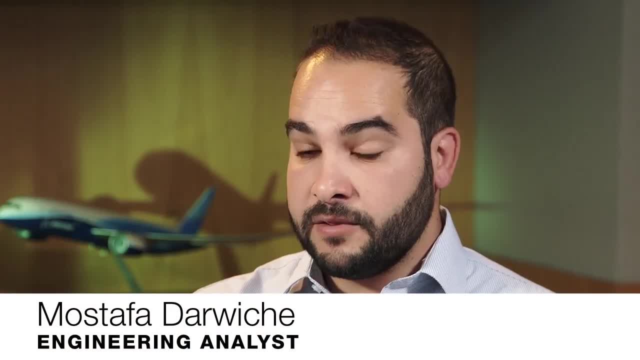 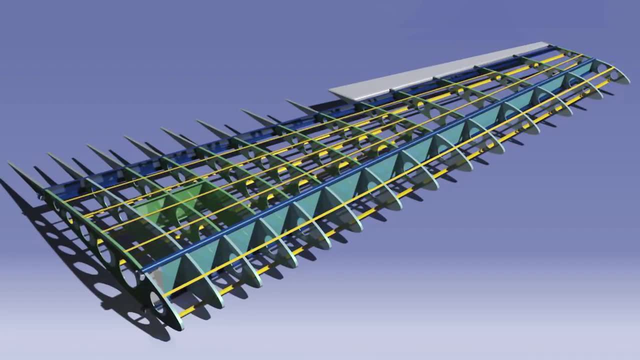 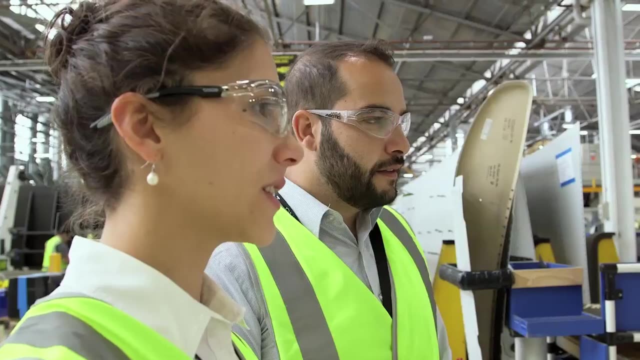 be flowing through that, and this involves modelling, using maths to model the structure, and we idealise something like a complex structure- say, a wing spar is something a lot simpler- into a beam that we can then use our maths to identify where the highest loads will be and design from there. 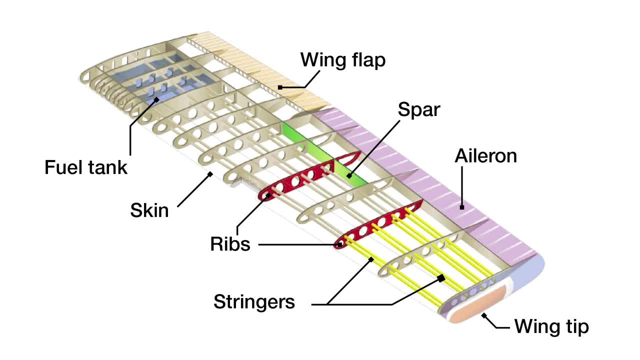 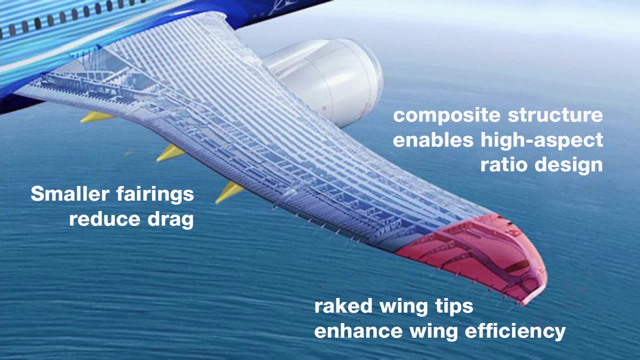 The internal wing structure consists of ribs, which give the aerodynamic shape, and the ribs are supported by the spars, which are simple beams that usually have a cross section similar to an I-beam. The spars are the most heavily loaded parts of an aircraft. They carry much more force. 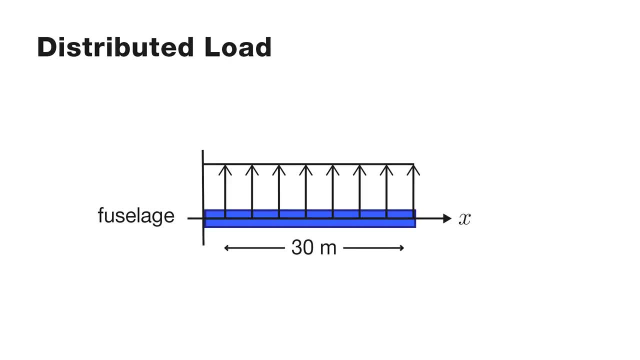 at its root than at the tip. The wing can be modelled as a beam with one end fixed to the fuselage. The three important qualities associated with the forces on the wing are the distributed lift load on the wing, the shear force and the bending moment. The beam is considered to be 30 metres long and 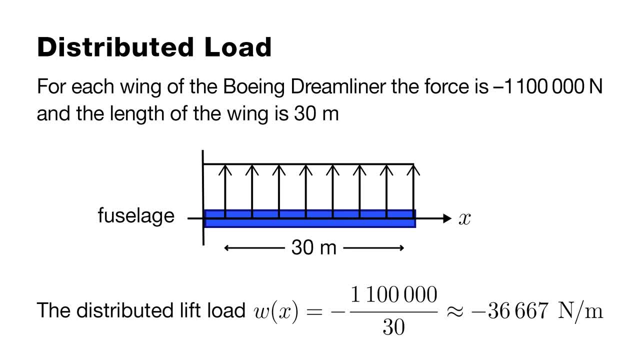 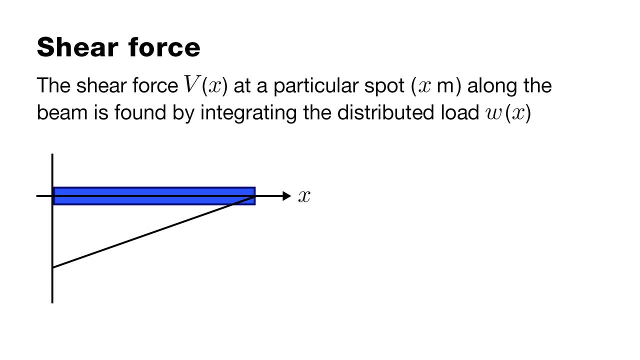 the distributed load is found by dividing the total force by the length. Shear force is the force in the beam acting perpendicular to the x-axis. For design purposes, the beam's ability to resist shear force is important. The shear force is at a maximum at the point. 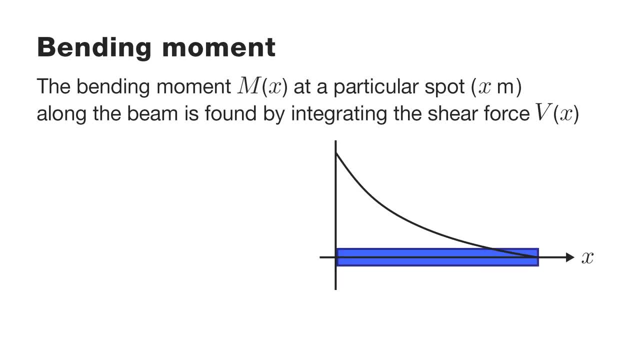 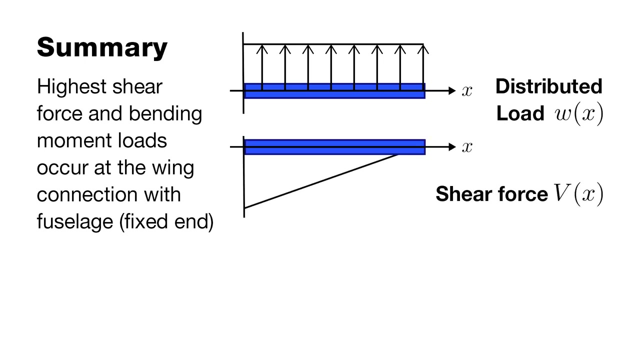 of the wing joining the fuselage. A bending moment is the reaction induced to the beam when an external force causes the beam to bend. A moment is calculated as the perpendicular force multiplied by the distance from the point. A bending moment is essentially the force that is applied to the beam when it bends. 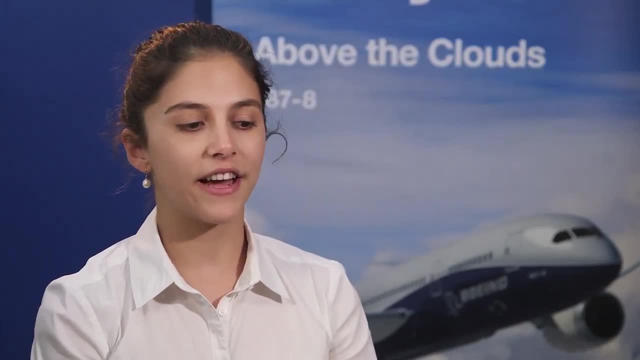 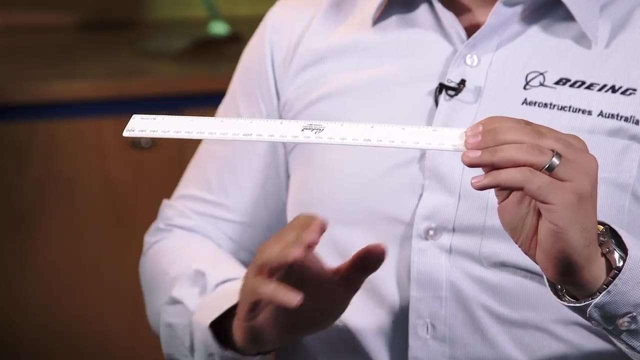 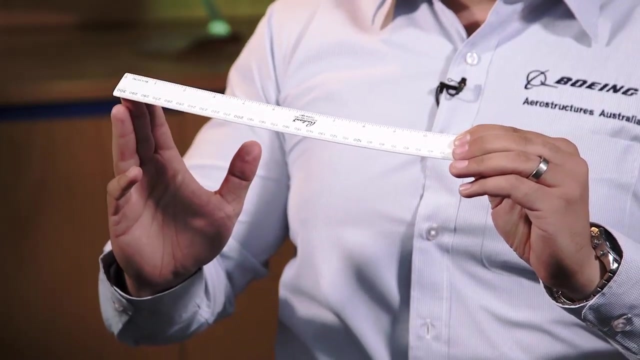 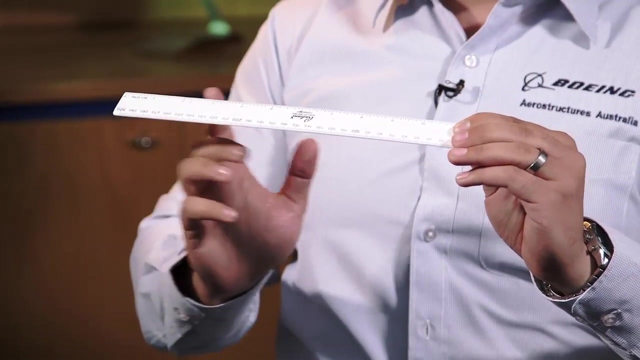 With a bending moment. the bending moment is theelle. A bending moment is the Village of the other�uffice of a horizontal energy mixture. If you assume that the bending moment applies to the fuselage and not the fuselage, ie where the handooping force or the fuselage would be, the bending moment is the compressiveness. 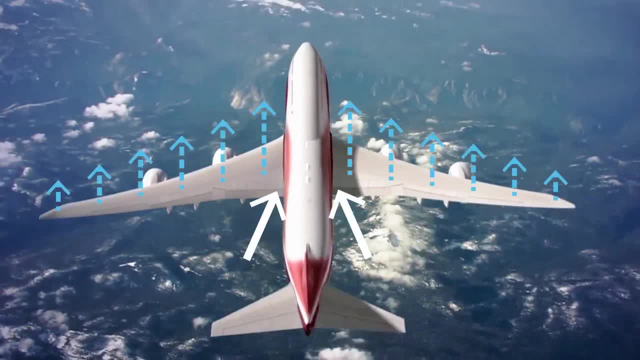 We determine the bending moment at various locations along the wing. Based on this, we know that the highest bending moment is going to be at this junction, at the fixed point, and this will then result in the highest stresses being at this point and therefore the most structure required in the beam, for example. 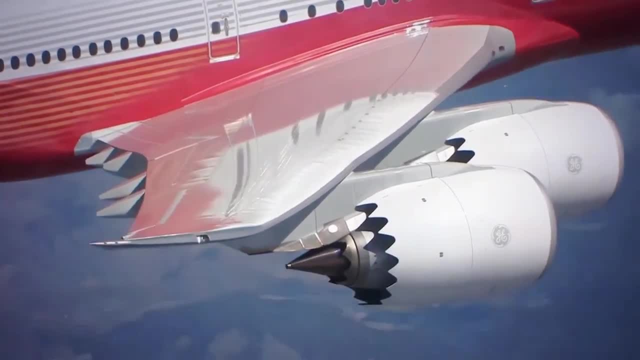 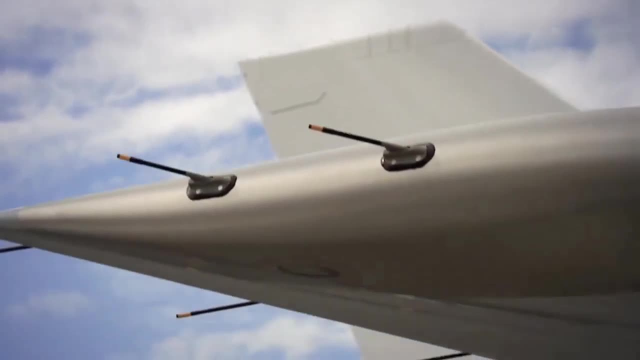 Designing a spar for a wing, we need to pick a cross-sectional shape for this beam that both maximises strength- the ability to carry bending- but also minimises weight. The second moment of area is a property of a two-dimensional plane shape. 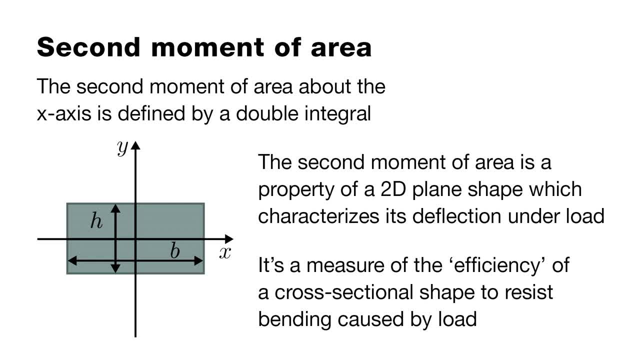 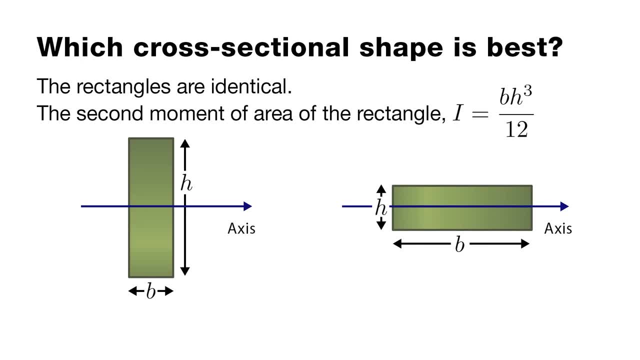 that describes its deflection under loading. It's a measure of the efficiency of a cross-sectional shape to resist bending caused by loading. Here are the moments of inertia for several shapes. Which shape has the largest moment of inertia and area to minimise the stress? 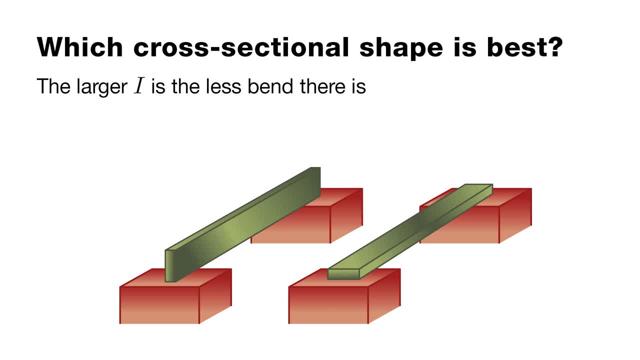 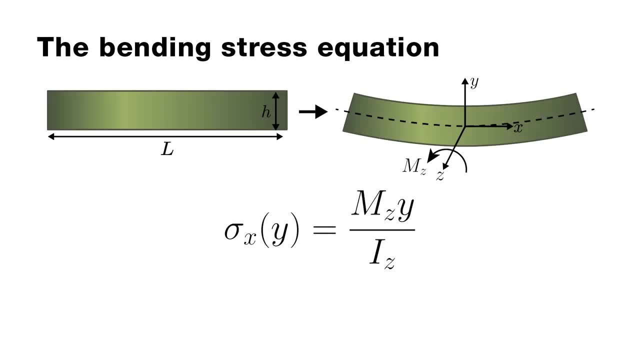 The larger I is, the less bend. there is An equation of the moment of area, and the moment of stress is the following: An equation is used to assess the strength of a structural element. It is known as the bending stress equation. The consideration of bending and stress is very important in wing design. 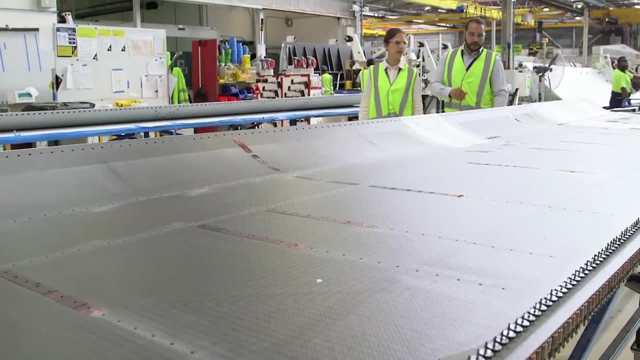 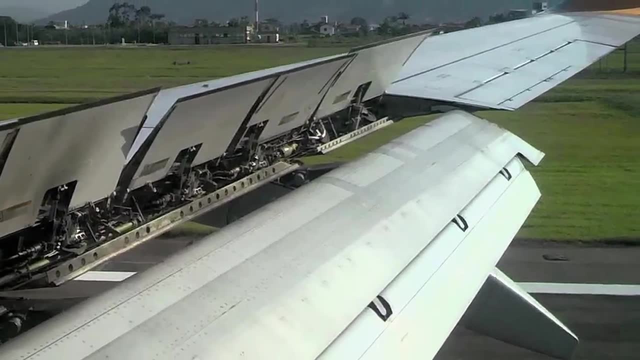 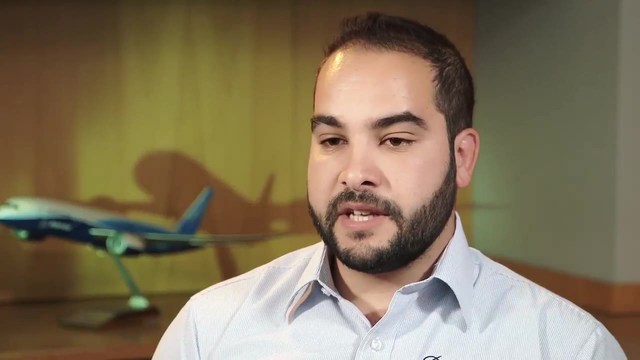 The movable trailing edge. the part built at Boeing Aerostructures Australia alters the shape of the wing to provide higher lift at lower speed. The majority of my work is on the movable trailing edge. What that involves is ensuring that the aircraft structure will be able to sustain.